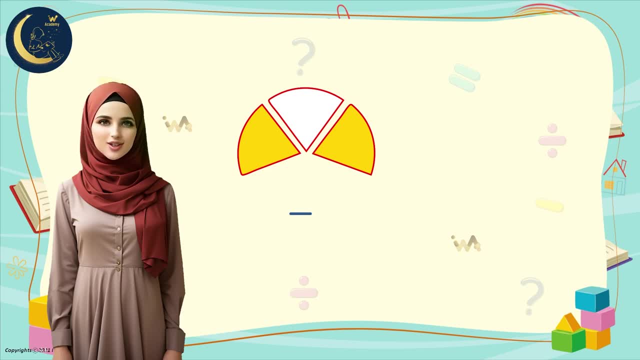 Two, You are great, So we will write here two. Now we will move to the denominator. What do we want to express here? Two, You are great, So we will write here two. Now we will move to the denominator. 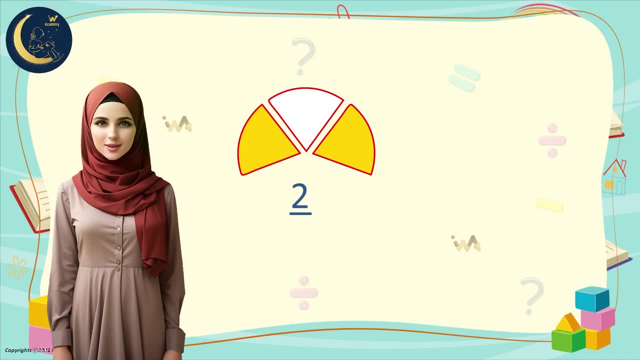 What do we write in the denominator? The number of all the parts. Well, how many parts do we have here? Three, You are wonderful, So we will write here three. We have two over three. What is the name of this fraction? 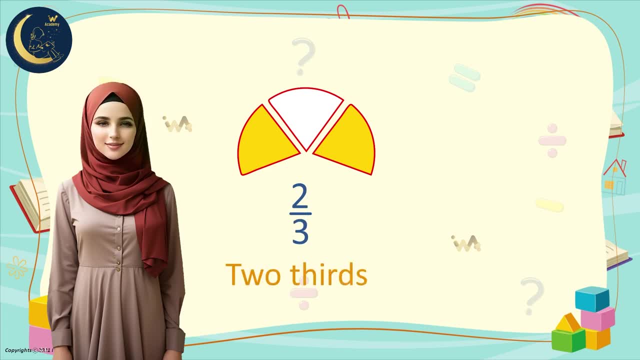 What is the name of this fraction? Two thirds. Its name is two thirds And it is written in the words like this. And it is written in the words like this: Two thirds. Well, let's see more shapes. Well, let's see more shapes. 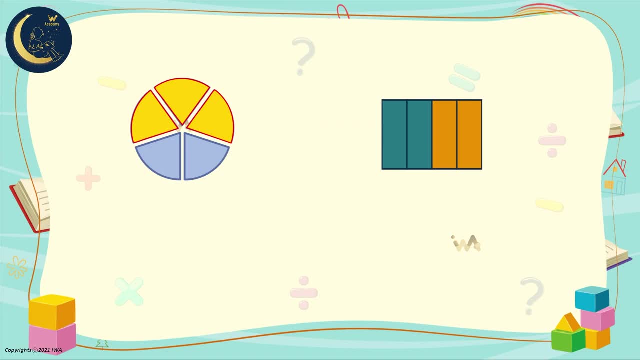 What is the fraction that expresses the colored parts? What is the fraction that expresses the colored parts? Let's start with this shape. First we will draw the fraction dash. What do we write in the numerator? What do we write in the numerator? 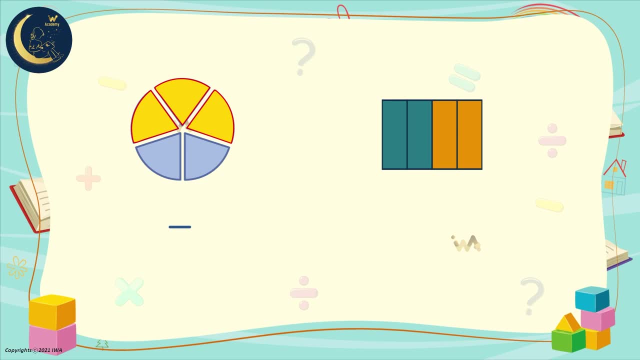 The number of parts that we want to express, Excellent. How many parts do we want to express here? How many parts do we want to express here? Three, You are great, So we will write here three. Now we will move to the denominator. 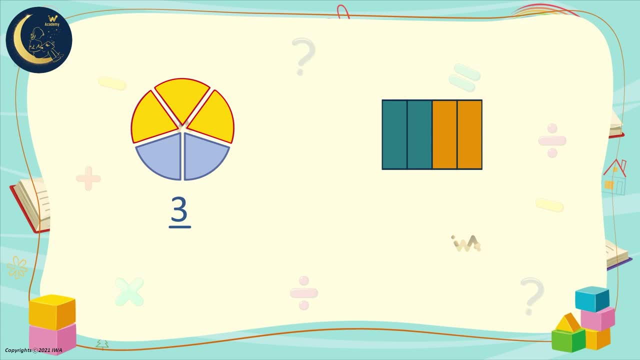 What do we write in the denominator? The number of all parts. Excellent, How many parts do we have here? Five, You are great. We will write here five. Now we have three over five. What is the name of this fraction? 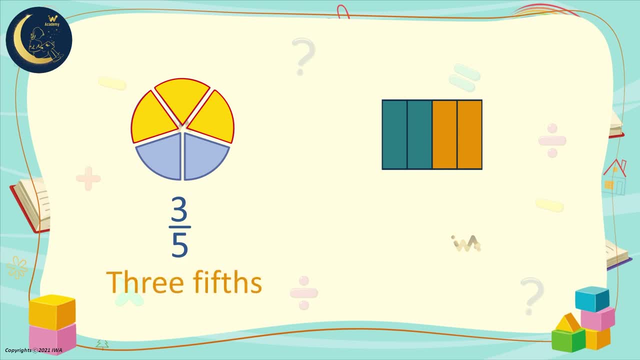 What is the name of this fraction? Three fifths? Its name is three fifths And it is written in words like this: Three fifths. Now we will write the fraction that expresses these parts. We will draw the fraction dash. 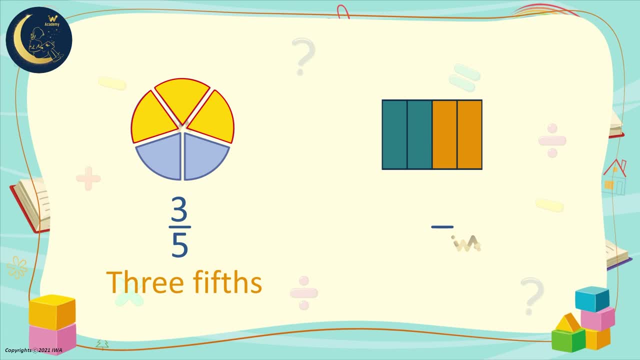 What do we write in the numerator? What do we write in the numerator? The number of parts that we want to express. The number of parts that we want to express. Well done, How many parts do we want to express here? Two: 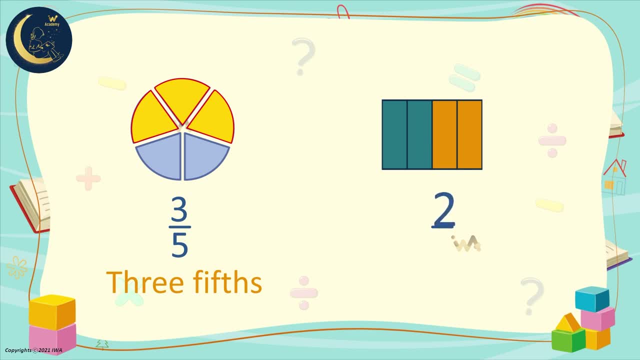 You are great, So we will write here two. Now we will move to the denominator. What do we write in the denominator? The number of all parts, all parts, Excellent. How many parts do we have here? Four, You are great, So we will. 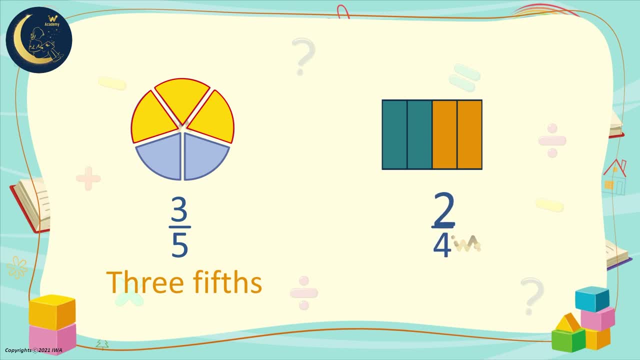 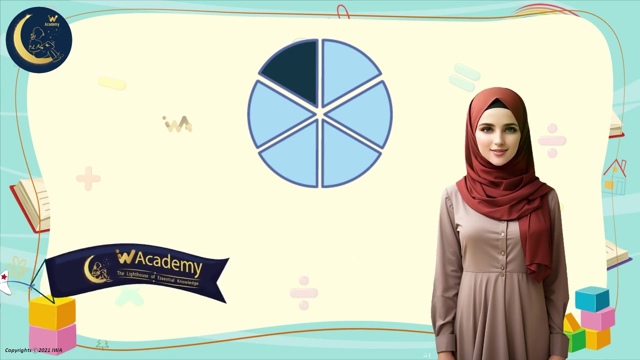 write here: four. Now we have two over four. What is the name of this fraction? Two quarters. Its name is two quarters and it is written in words like this: Two quarters. Good job. We want to express the colored parts in this shape, with the appropriate fraction. 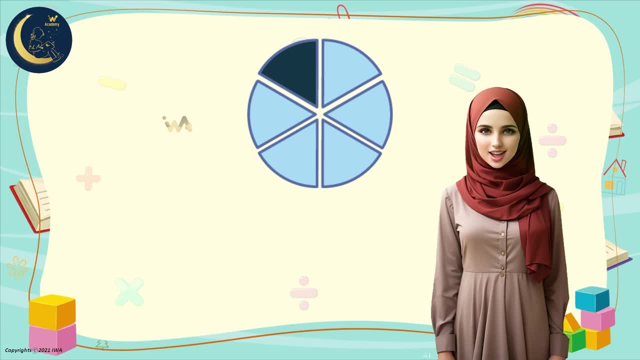 Look, this shape is made of six parts. okay, First we draw the fraction dash. What do we write in the numerator? The number of parts that we want to express. Excellent, How many parts do we want to express here? One, You are great, So we will write here one Now. 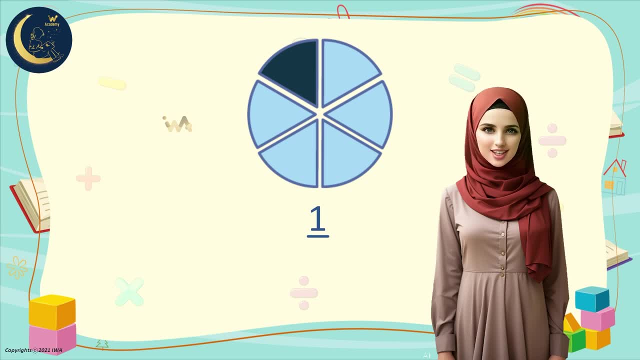 we'll move to the denominator. What do we write in the denominator? What number do we write here? One One, So we have two over four, You are great. So we have two over denominator. The number of all parts. Well, how many parts do we have here? Six, You are. 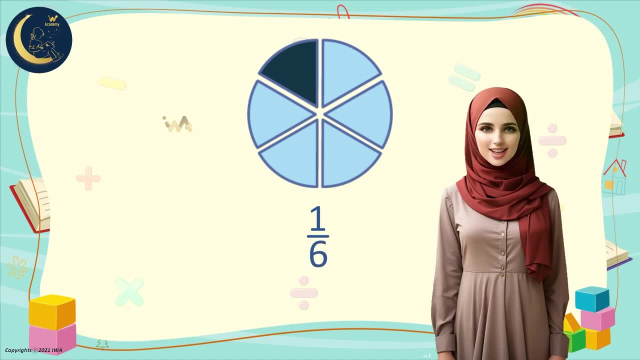 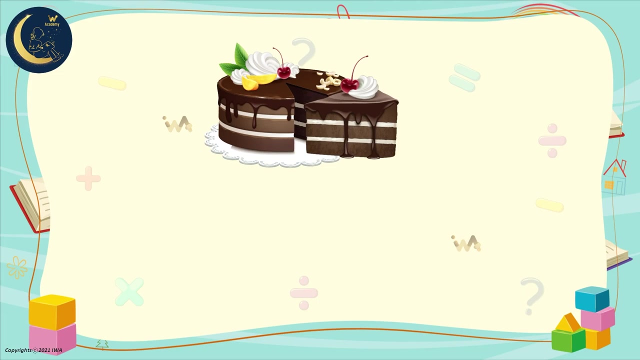 great. So here we will write six. Now we have one over six. What is the name of this fraction? One sixth? Its name is one sixth and it is written in words like this: One sixth. On your birthday, your mother divided the cake to seven parts and you got one of these parts. 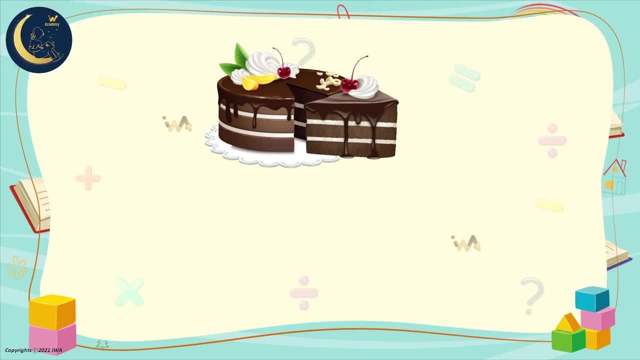 Can you write the fraction that expresses the part you got? Excellent, First, we will draw the fraction dash. What do we write in the numerator? The number of parts that we want to express. Well done, How many parts do we want to express here? One, You are great. 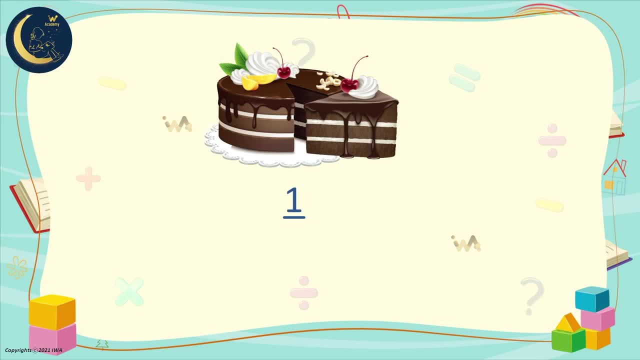 So here we have one. sixth, What is the name of this fraction? Six, You are great. So here we will write one. Now we will move to the denominator. What do we write in the denominator? The number of all the parts. Excellent. How many parts do we have here? Seven, You are. 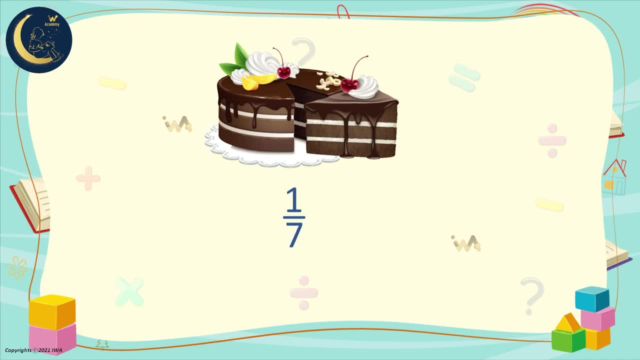 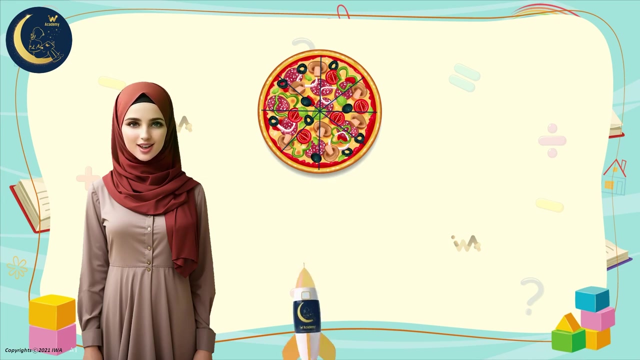 great, So here we will write seven. Now we have one over seven. What is the name of this fraction? One seventh? Its name is one seventh and it is written in words like this: One seventh. What a delicious pizza. It was divided to eight equal parts and you got a piece, Can? 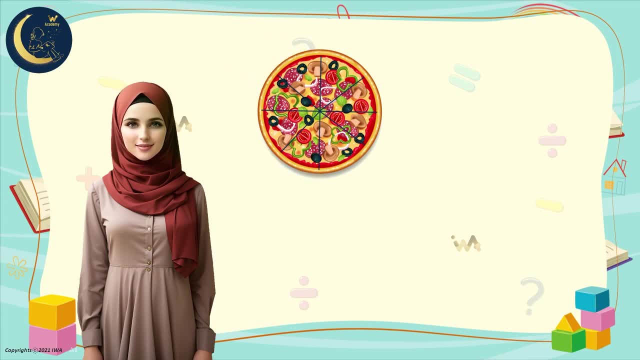 you express the part that you got by fractions. Well, first we draw the fraction dash. What do we write in the numerator? The number of parts that we want to express. Well, how many parts do we want to express here? One, You are great. So here we have one. sixth, What? 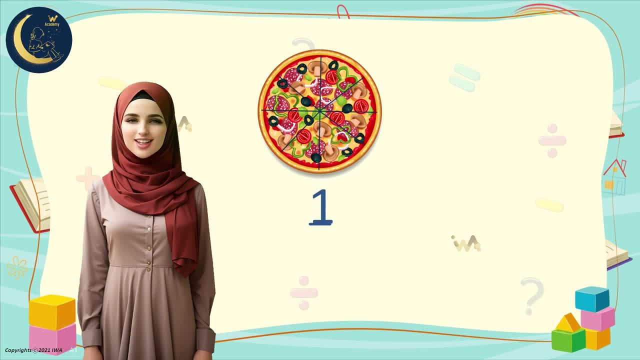 is the name of this fraction One eighth. Its name is one eighth and it is written in words like this: So here we will write one. Now we will move to the denominator. What do we write in the denominator? The number of all parts. Excellent, How many parts do we have here? Eight You. 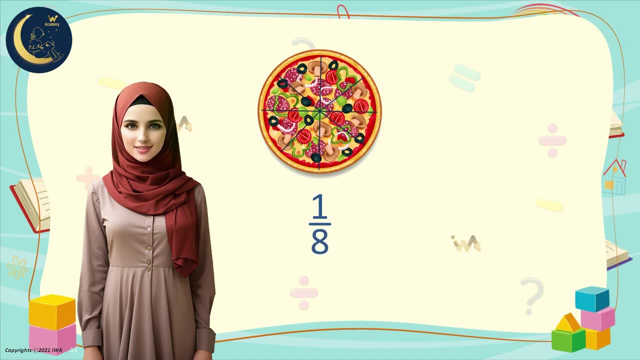 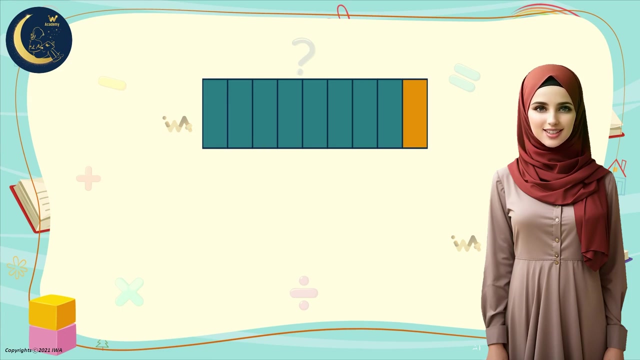 are great. So here we will write eight. Now we have one over eight. What is the name of this fraction? One eighth? Its name is one eighth and it is written in words like this: One eighth. This shape is divided to nine equal parts. Who can tell me how to express? 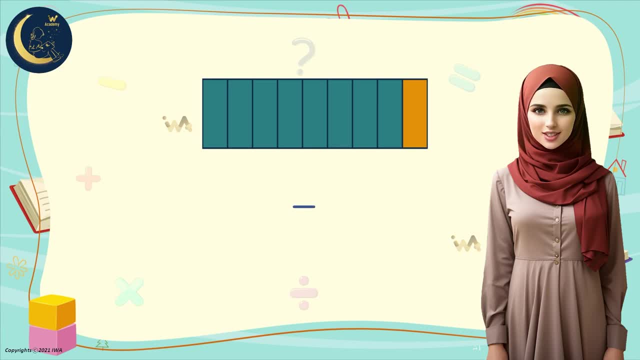 this part Excellent. First, we draw the fraction dash. What do we write in the numerator? The number of parts that we want to express. Well, how many parts do we want to express here? One, You are great, So we will write here one. Now we. 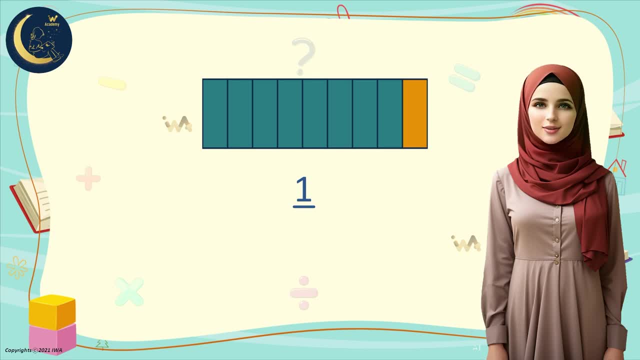 will move to the denominator. What do we write in the denominator? The number of all parts. Well, how many parts do we have here? Nine, You are good. So we will write here nine. Now we have one over nine. What is the name of this fraction? One ninth Its name. 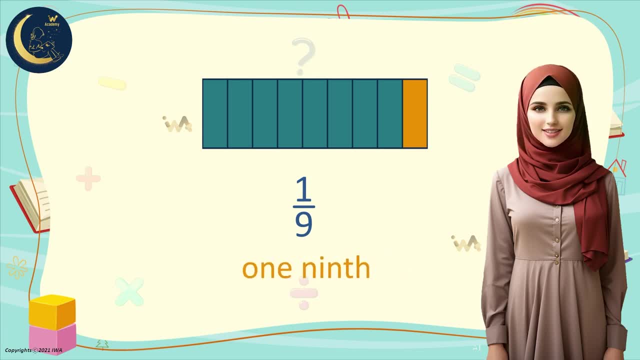 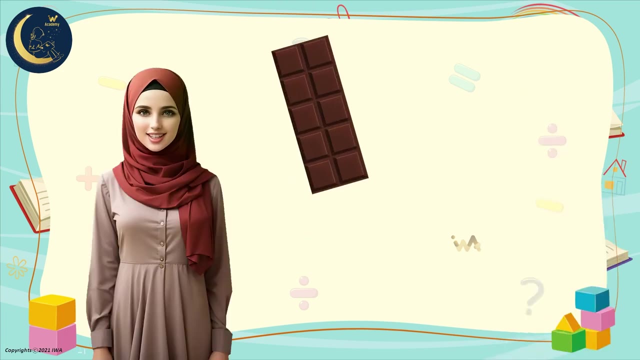 is one ninth and it is written in words like this: One ninth. In this part we also have to express as one ninth and this two. The result of adding all these parts is one. Look at this chocolate. It is divided to ten equal parts. How can we express this part using?